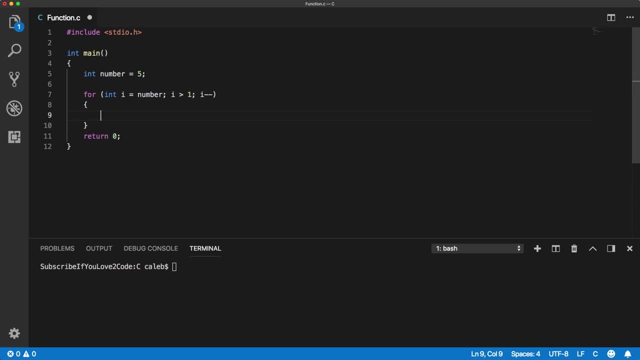 Then we decrement And then what we can do is we basically keep track of what the number is. So let's just start with 1.. The reason I'm using 1 is because we're multiplying. If we set it to 0 and started multiplying, we wouldn't get any value. 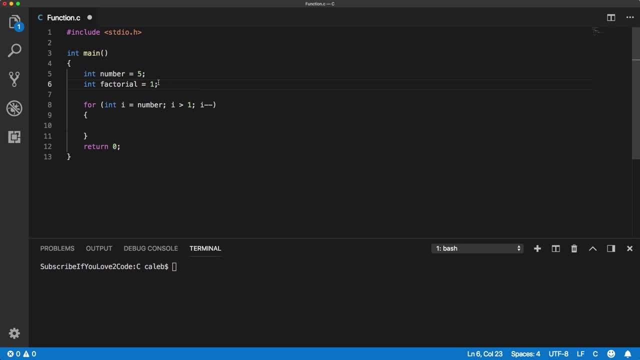 So 1's not going to change the multiplication at all, but it's going to allow us to actually keep track of the value that way. So we might do something like this: Factorial, And then we're going to multiply that by i. 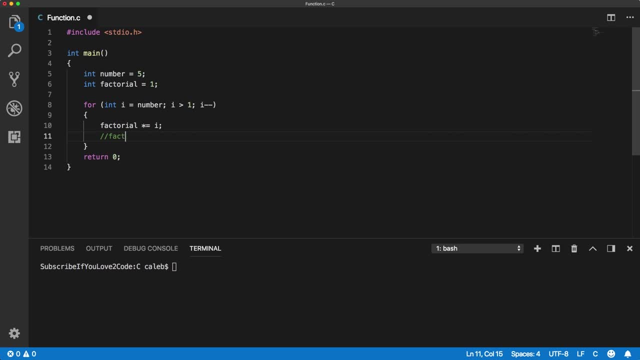 So if you guys aren't familiar with this, this is the same thing as doing just a shorthand, So you can put the multiplication on the left hand side of the equal sign. So what's going to happen is i is going to be 5 and we're going to do 1 times 5, and then it's going to decrement down to 4.. 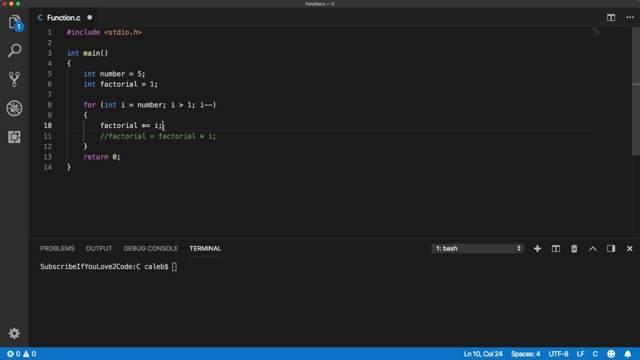 We're going to do whatever that value is. Well, it's going to be 5.. 5 times 4. Times, 3. Times, 2. Times, 1. And so forth, And then, at the end, we're going to print that value. 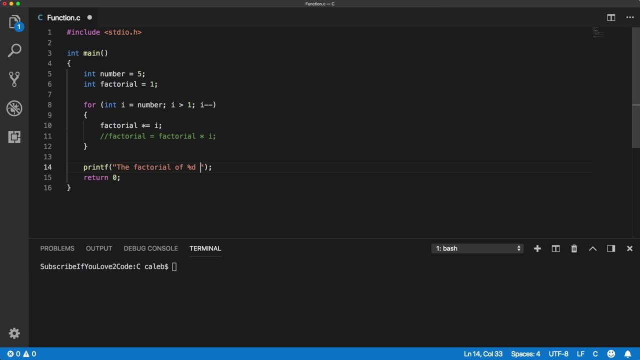 And we can say: the factorial of the number is the number, So number is the number we're asking for, the factorial of, and then factorial is the actual result, And then we can return 0.. The program's done, So let's try it out. 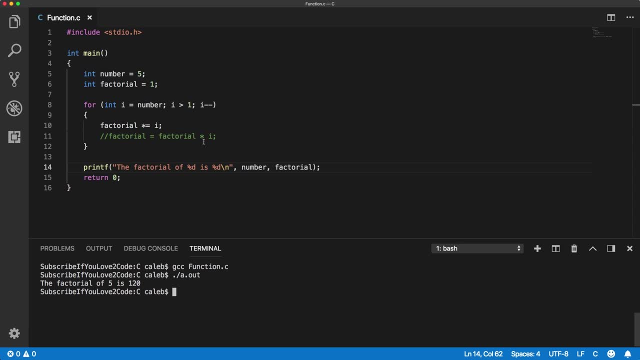 The factorial of 5 is 120.. So it seems to be working. But now the issue is: you know what, if we wanted to calculate the factorial of- I don't know- 20. The factorial of 120. And we just wanted to. well, that's a really big number. 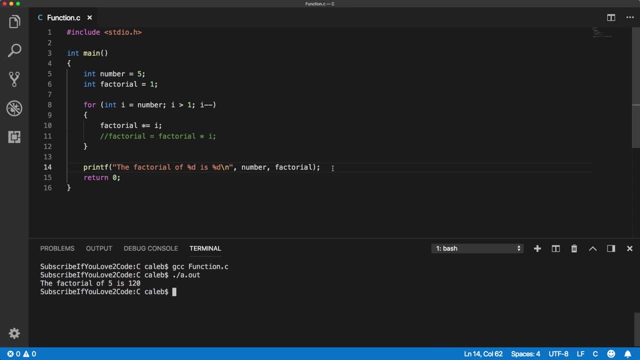 And we just wanted to keep doing it until we got tired of calculating the factorial. Well, we might have to go in here, We might have to change this hard-coded value, And then we'd have to keep running the program. And you know, it's just not very scalable, right. 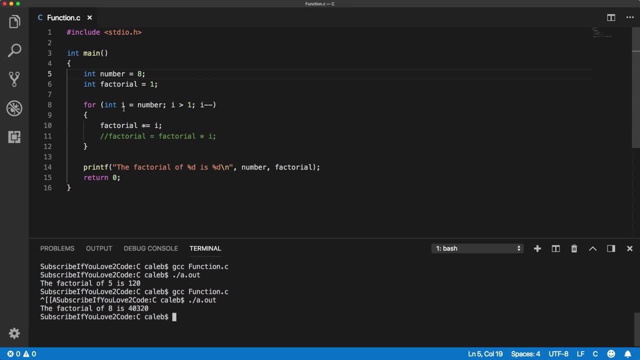 And especially if you wanted to calculate the factorial twice in one program, you'd have to basically copy all this code and paste it below and then change some things, And it's just really not that good. So this is where there's a huge red flag that we might want to create a function. 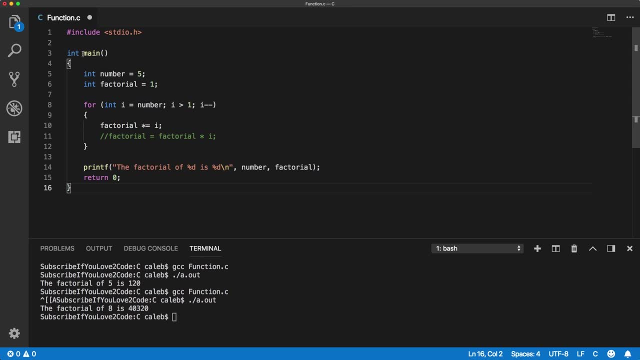 Now, if you look at main, this is actually a function And we're going to basically create another function So we can kind of follow the format of main. So it has a data type. This is what's known as the return type. 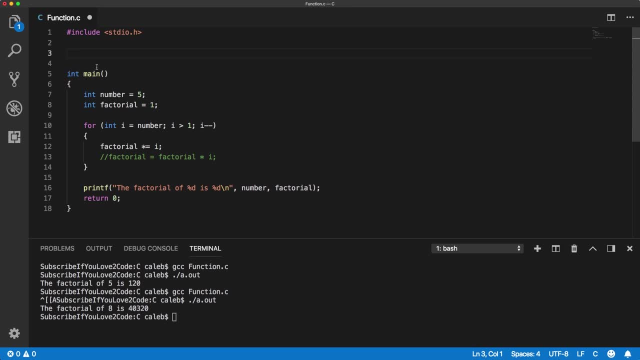 And that is the value it gives back. So you can think of the function as basically something we throw some data at and it throws some data back. It does all the work for us. We don't have to do anything, We just have to create it. 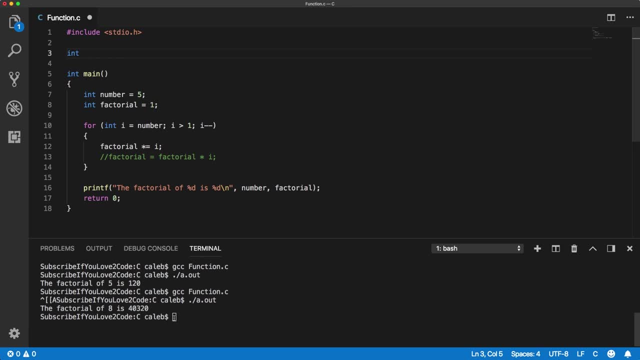 So it's going to create, it's going to return an integer, because the end result right here is an integer And it's always going to be an integer when we're calculating the factorial Because, like I said in the previous videos, integers, times integers- always give you integers. 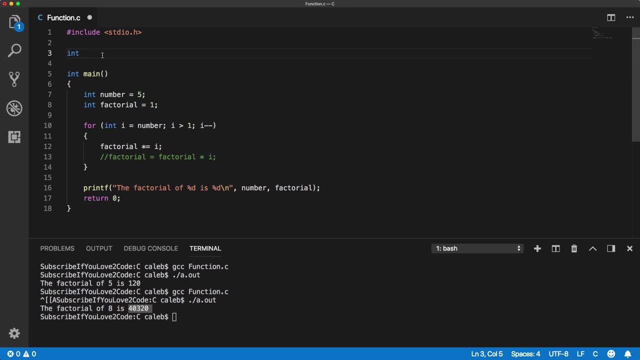 That's a concept known as closure. So it's going to return an integer and we can just call it factorial. So this is the structure, But so main doesn't have anything in these parentheses. I think you can put some stuff in there if you want to take like command line arguments or whatever. 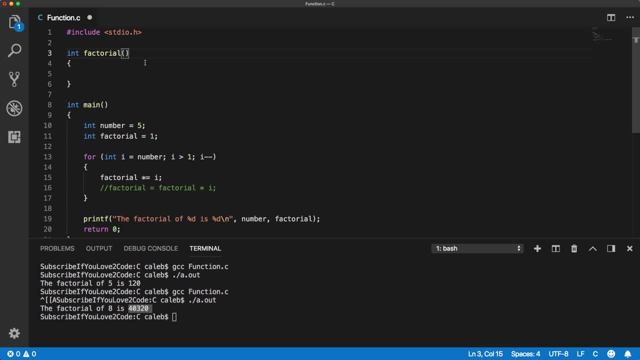 But for factorial, we definitely want to take something as a parameter, take it as an argument and store it in a parameter, So it would look something like this number. So this is the equivalent to this. What are we trying to calculate the factorial of? 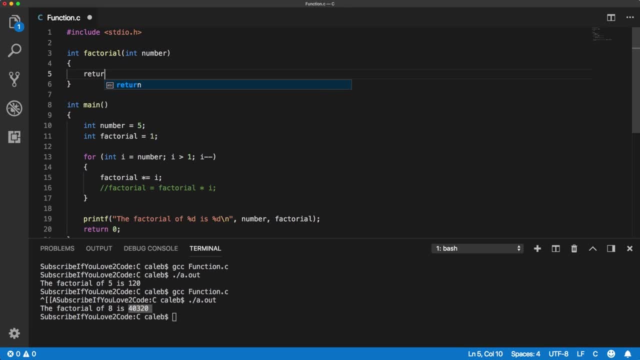 And then we're going to do is we're going to return the result, which is going to be factorial, And we need to declare that up here, just like, just like we're continuing from right here. So So we start with one and then we go through the process of this multiplication. 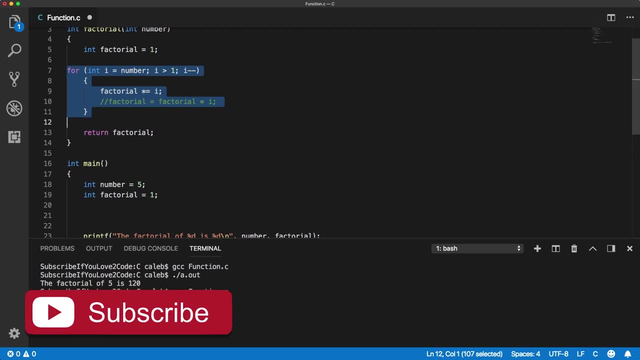 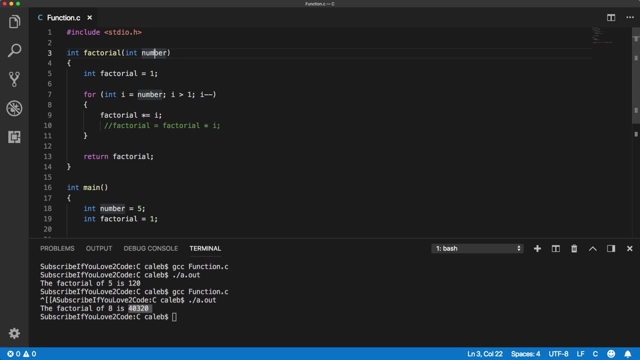 All right. So now I think our function works because we have the number and we have the factorial. All the other code works exactly the same. Now, in the next video, I'm going to be talking about how we call this function and how it would be different than having, how it would be different than having the code in main, and what we need to change to make everything work right. 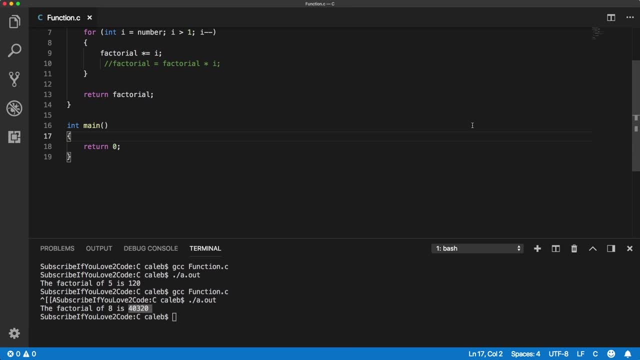 So. So thank you guys for watching. Be sure to check out the next video. Appreciate you watching and please be sure to subscribe If you've enjoyed the series. Also, check out the link for a link to check out the description, for a link to my C programming crash course.